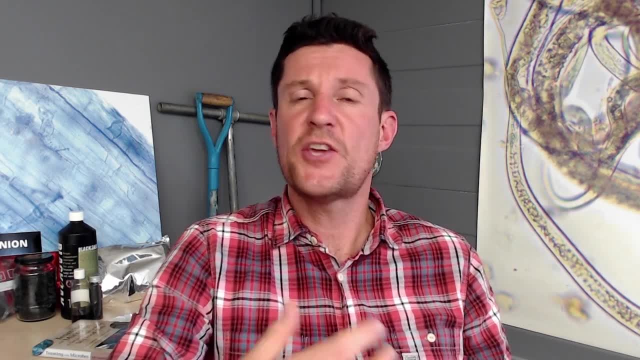 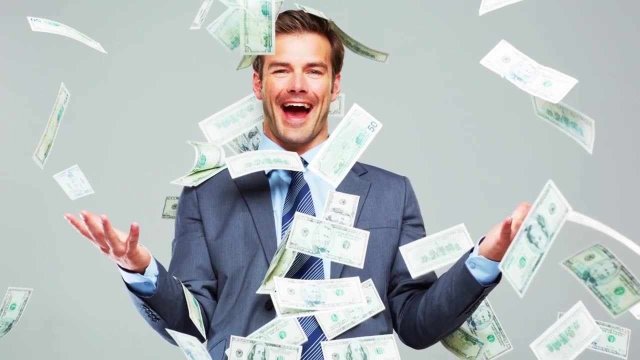 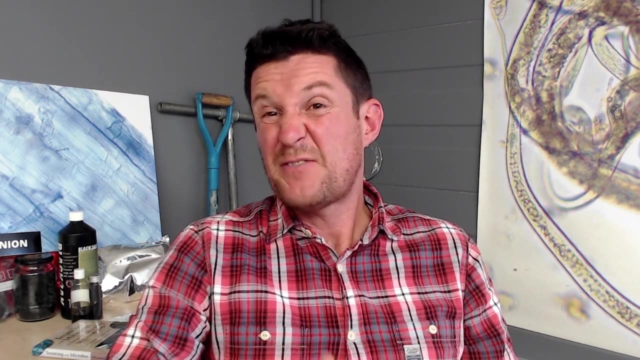 of funding or funding streams, and we should all understand that a huge proportion of scientific research is funded by those who stand to financially, benefit or not from the information one way or another. So it might also be that the subject matter is just not interesting enough to 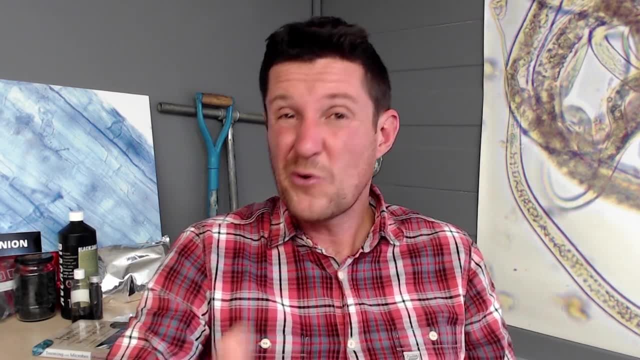 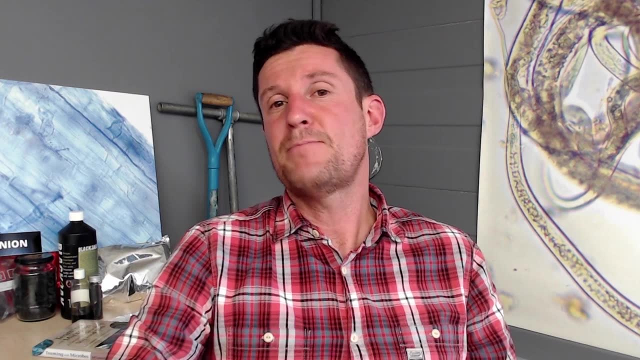 new scientists or those already engaged in other projects. Soil has only recently really become more and more important, So it's a lot of work to do. So it's a lot of work to do, So it's a lot more sexy. So, whatever the reasons, there is simply not a lot of evidence out there that you can find. 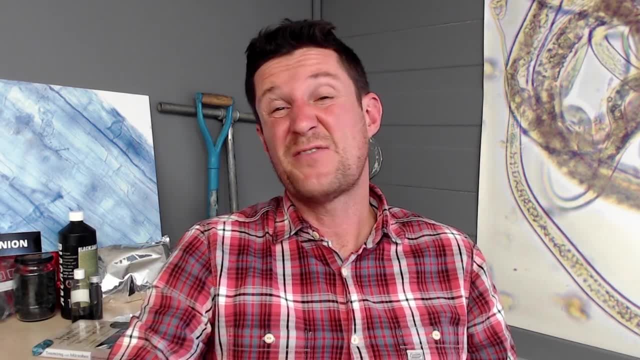 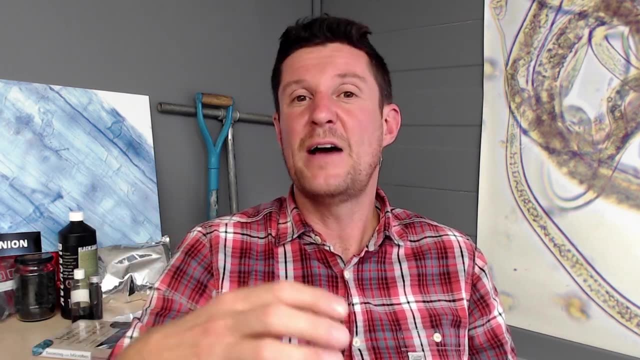 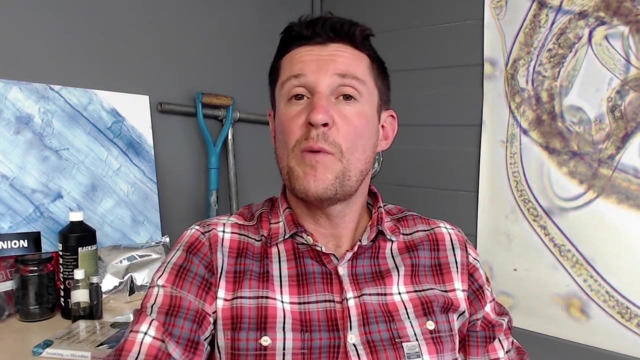 on the internet, and the little that does exist actually does very little to match up the evidence with the increasingly popular belief that soil microbial balances are important, And this is not really very helpful to us. Now just to clarify: when we talk about organism ratios we're referring to 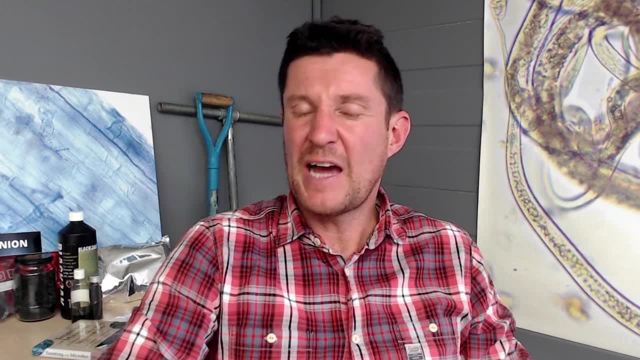 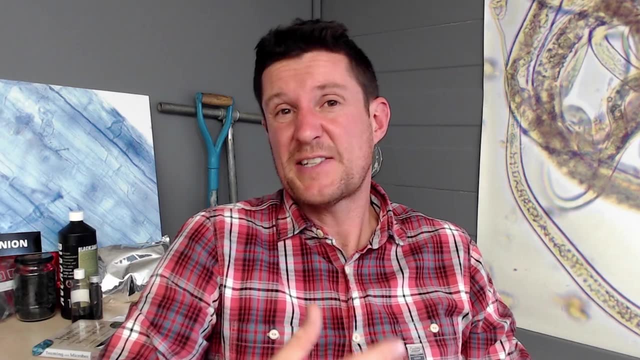 the amount of each type in relation to the type of soil that we're talking about. So we're talking about the amount of each type in relation to another. In most cases, this is about bacteria versus fungi, And we're not actually concerned with the numbers of each of them, although this does have an 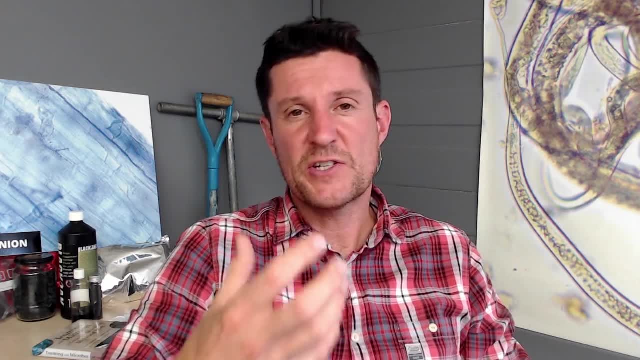 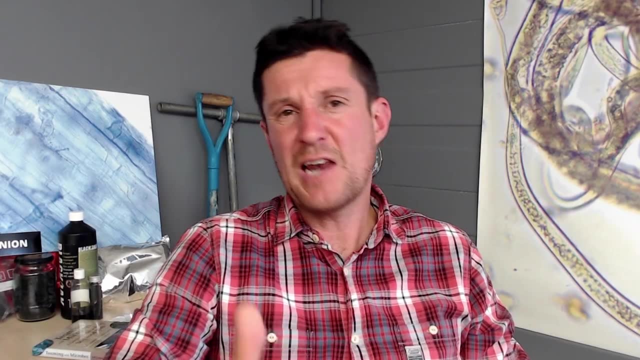 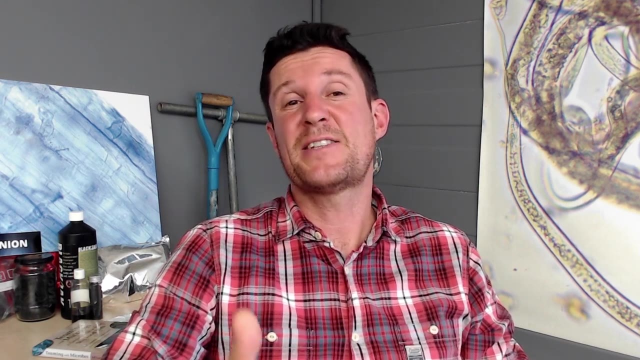 impact on the output. What we actually are concerned with is the mass of each in relation to each other, So what we refer to as the biomass. Due to the scale of these little critters, it's clearly going to take a lot of bacteria to make up the same mass as fungi, And so the way in which you 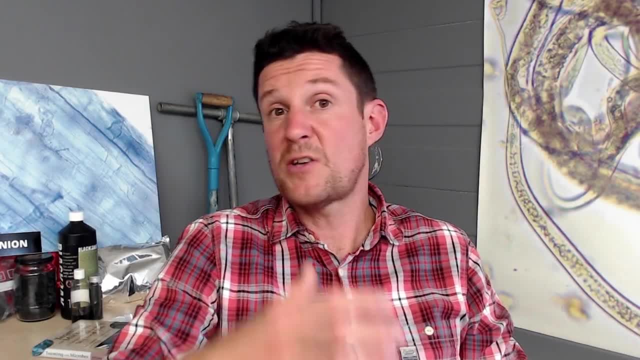 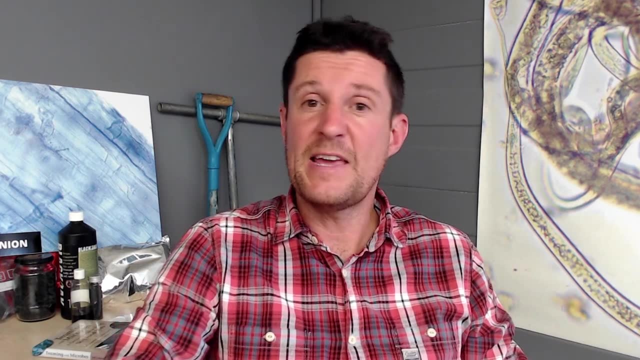 measure these organisms and determine your biomass has also compounded this issue in the lack of evidence And there's numerous ways to calculate biomass of bacteria and fungi and the associated ratios with that, If people do this differently, which they have in many of the studies I looked at, 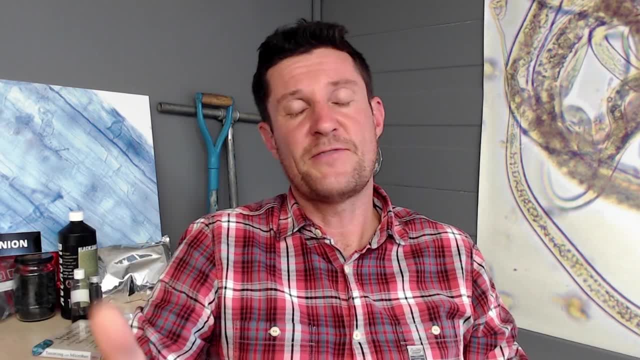 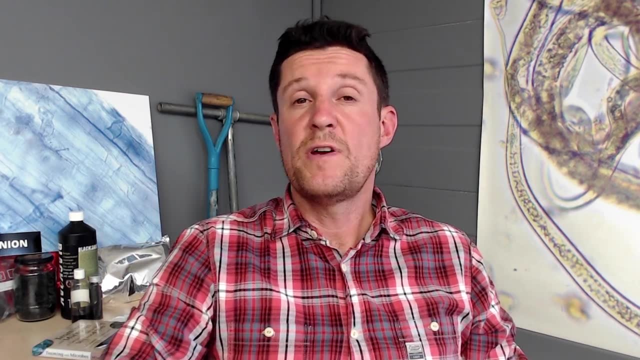 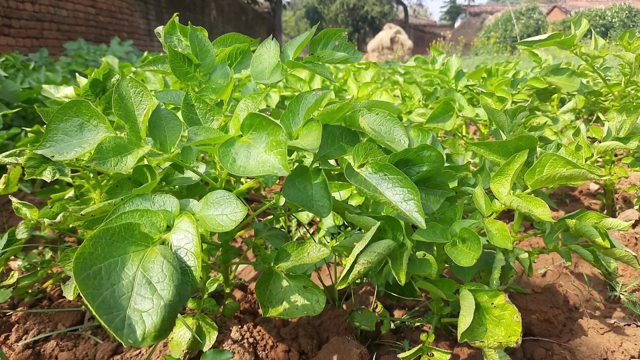 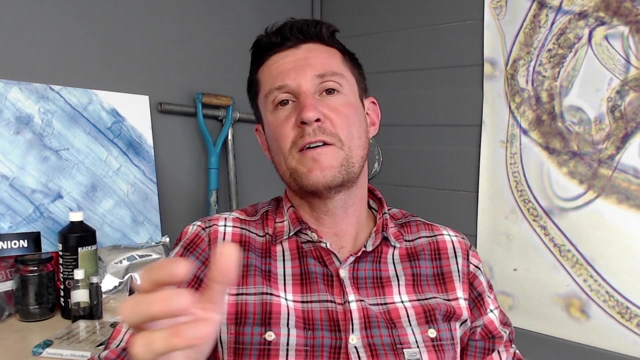 then the results will also be different as well, And that again doesn't really help things. But all plants are key drivers of soil processes. They communicate, stimulate and interact with all the organisms that they want in the soil, And those organisms will work for them. Now, with all of this, being known. do you really need to build soil life and adjust the balance of bacteria compared to fungi to be more optimal for your plants? After all, we know, woody shrubs and berry fruit prefer more fungal soil, and trees don't have as much fungal soil as they do, So we're going to have to. look at what plants do as well. whereas grass is thriving, more bacterial soil. So can't the plants do all the work for us? Won't they create their own optimal soil conditions? Well, the answer is actually partly yes. They can do a lot of the heavy lifting for us, but perhaps not all. What happens if you're dealing?